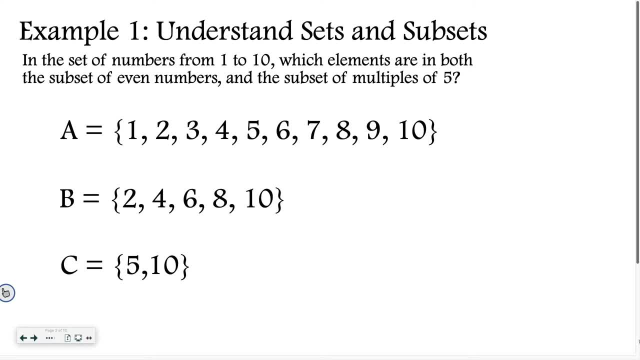 in the set of numbers from 1 to 10, so that means all of the numbers between 1 and 10.. In this case we're just talking about integers, whole numbers, so none of the decimals. So a right. here is our set of numbers, 1 from 10.. Which are elements, so vocab word, each of these. 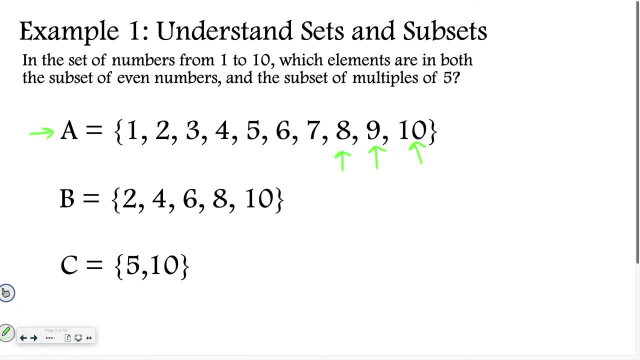 numbers is considered an element in the set. So the whole thing here is a set, and then each individual number is an element. So a set is the whole thing, an element is each individual thing. All right, so in the set of numbers from 1 to 10, which elements are in both the subset? 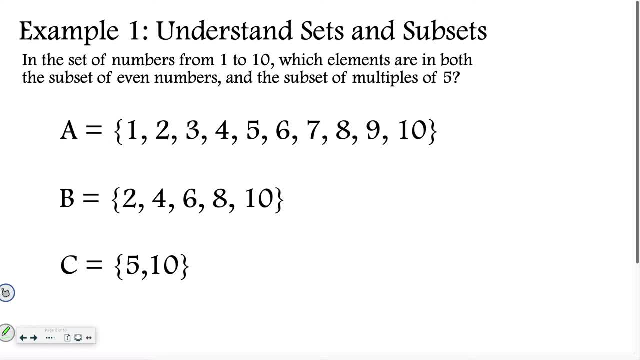 of even numbers and the subset of multiples of 5?? So a subset is when you take the set and you pull out a smaller group. So the subset of even numbers would be 2,, 4,, 6,, 8, and 10.. 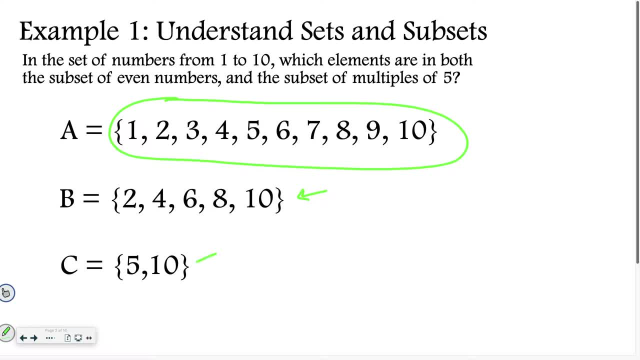 The subset, that is, the multiples of 5, out of the numbers 1,, 2,, 3,, 4,, 5,, 6,, 7,, 8,, 9, and 10.. The only ones that are multiples of 5 would be 5 and 10,. okay. 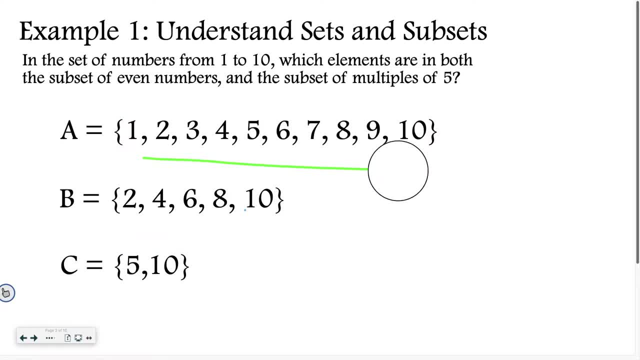 So we have our set. Set A is all of the numbers right. Set B is a subset of set A. It's a smaller version of set A, And C is a subset of set A. It's a smaller version of set A, And we want to know. 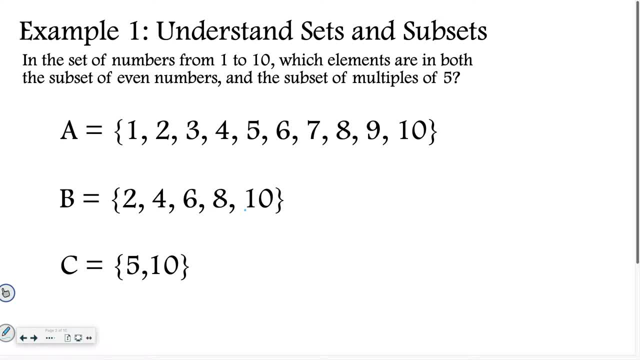 which elements are in both subsets. So 2 does not appear in both, 4 does not appear in both, 6 does not appear in both, 8 does not appear in both, But if I look, 10 appears in both. 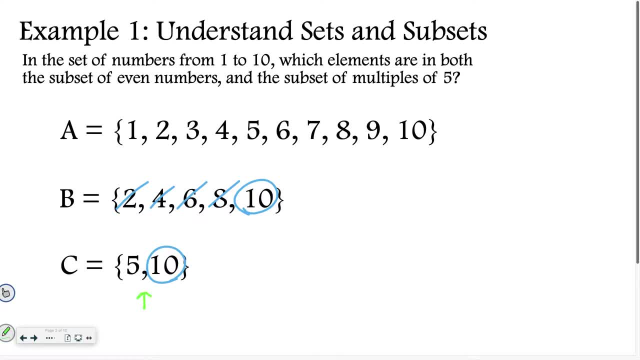 Or a faster way would have been to start with the smaller set, be like there's no 5 in the other one, but look, there's a 10, and I would have been done So. all this question was asking was which number appears in both sets, And the answer would be the number 10.. 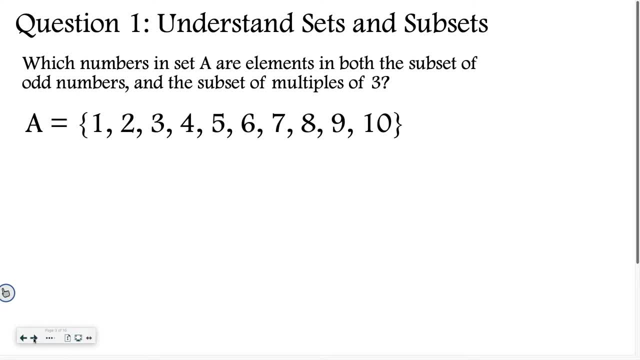 So that means it is your turn. Question 1 for you: which numbers in set A- so I've listed set A for you- are elements in both the subset of odd numbers. So what you should do is you should make a subset B of the odd numbers and then the subset of multiples of 3.. So then 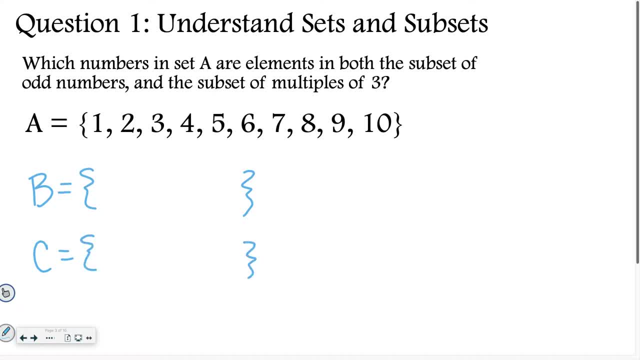 make a third set of multiples of 3, and see what numbers overlap between those two sets. Good luck Alright. hopefully you said the answer was both 3 and 9.. You saw that 3 is an odd number and it's a multiple of 3.. 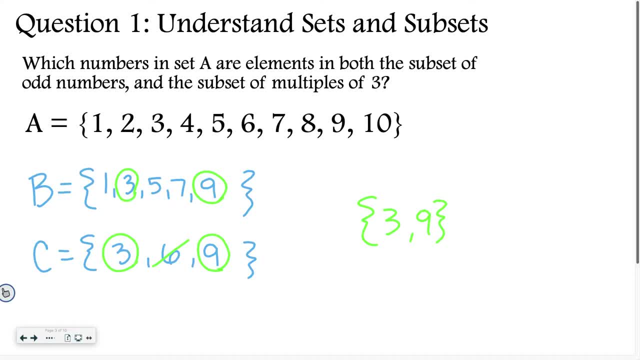 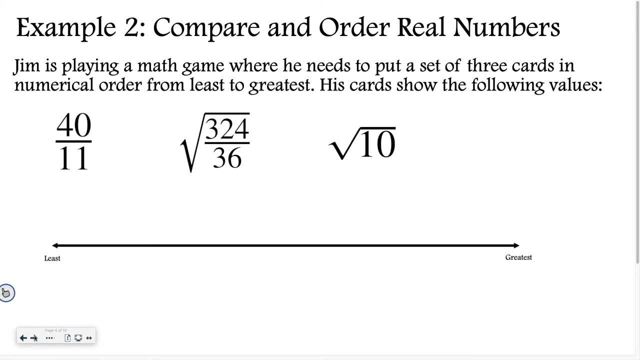 9 is an odd number and it's a multiple of 3. So you should have listed both of those answers. Now, example 2, compare and order real numbers. Jim is playing a math game where he needs to put a set of 3 cards in numerical order from least to greatest. 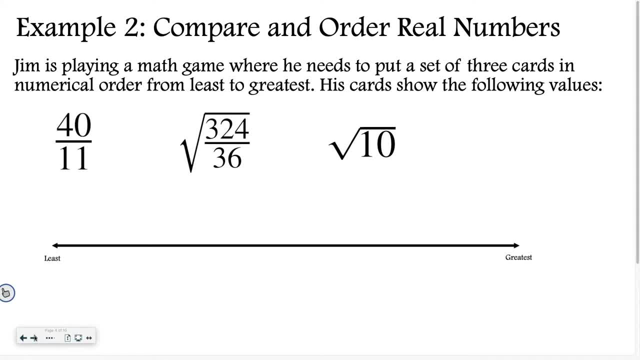 Okay, Big one. Long way of saying. we're ordering from smallest to biggest or least to greatest. Okay. His cards show the following values: 40 elevenths, square root of 324 over 36, and the square root of 10.. 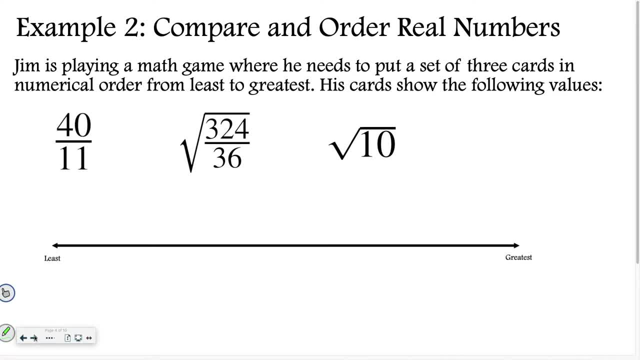 Now if you're looking at these and you're like I have no idea what these numbers equal, I would say you guys are most comfortable with decimals. At this point, you guys are probably the most comfortable with that. So what I'm okay with you doing is grabbing a calculator and saying: 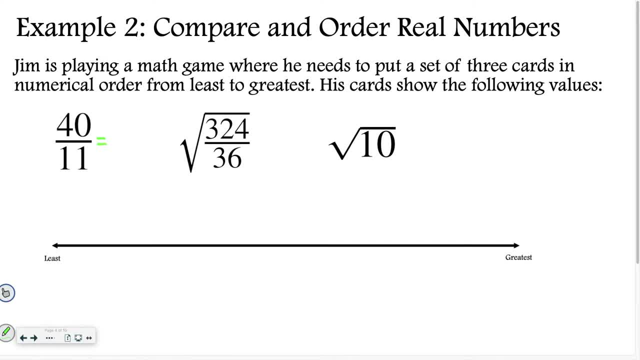 what is 40 divided by 11?? That is about 3.64.. Then in your calculator type in: what is the square root of 324 divided by 36?? When you do that, you should get 3.. And yes, even though I'm writing the answer on the board, you should be testing this to make sure you're using your calculator correctly. 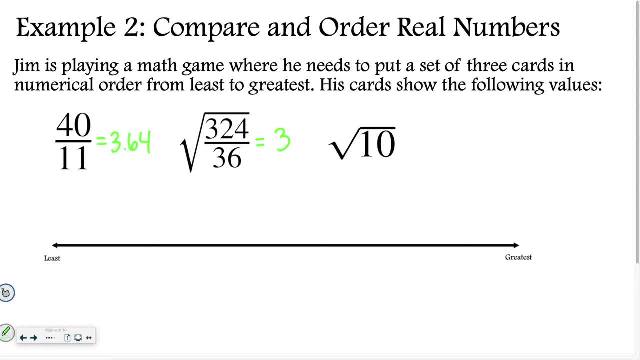 Because if you're not using your calculator correctly, you're not going to pass the test. if this is how you're doing these problems, right, So test it out now, when the answers don't matter. That way you can ask me questions if you need help. 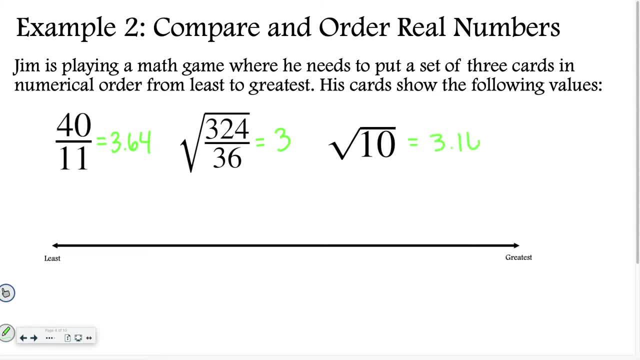 And the square root of 10 is 3.16.. So if I want to order these from least to greatest, my smallest number would be the square root of 324 over 36.. The next smallest number would be the square root of 10.. 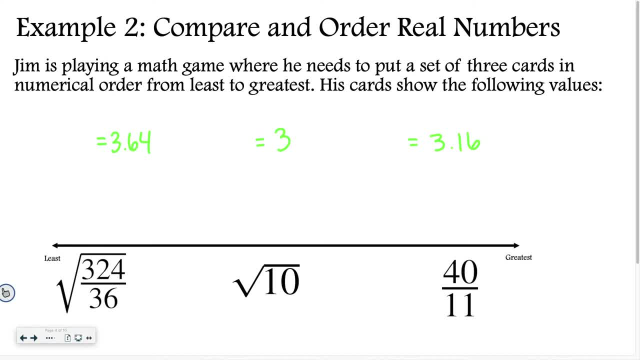 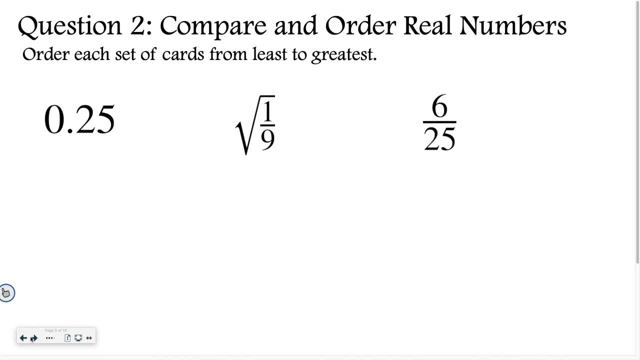 And the largest number would be 40 over 11.. So when you do this next question on your own, I suggest maybe checking out some decimals. Good luck, Alright, for this problem. hopefully you ended up with the smallest being 6 over 25, or 6 twenty-fifths. 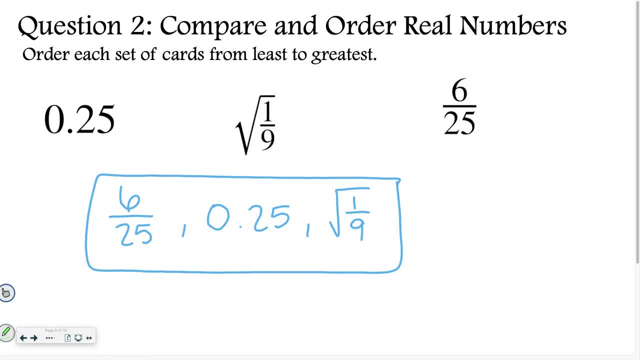 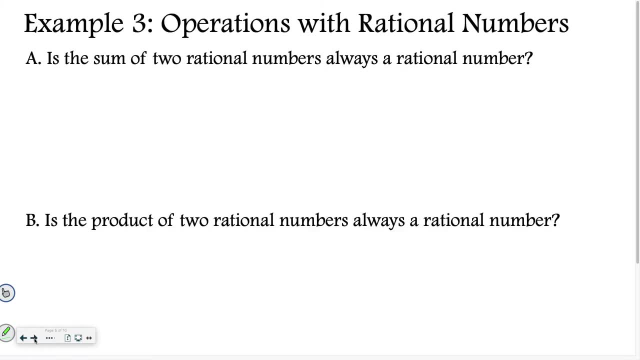 The second smallest being 0.25.. And the biggest, or I guess the third smallest, square root of 1 ninth. If you have questions about that, please be sure to ask for some help. Alright, example 3, operations with rational numbers. 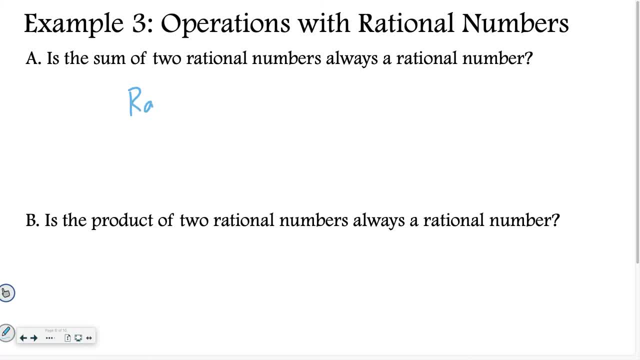 So let's quickly review. A rational number is any number that can be written as a fraction or decimal, And this includes repeating decimals. Irrational means that a number is non-repeating and never-ending, So that number goes on and on forever and ever. 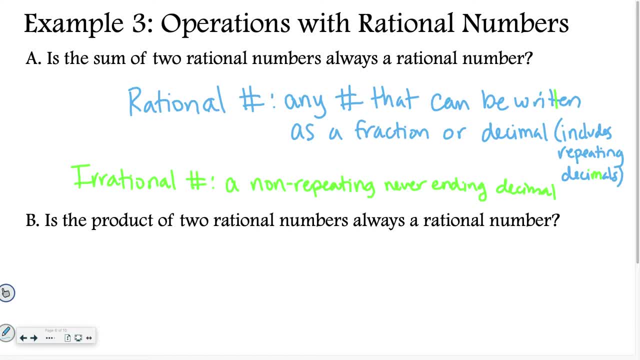 just like how you guys feel about my math videos. sometimes So irrational relates to Ms Johnson's math videos. They feel like they're never going to end So rational. Any number that can be written as a fraction or decimal includes repeating decimals. 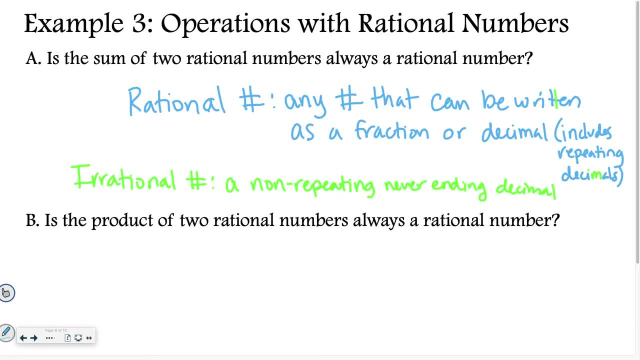 Irrational is a non-repeating, never-ending decimal. I'm going to erase this. so if you want to write that down, you should write that down before it disappears off the screen, or rewind the video and copy it down, Because we are going to look at letter A. 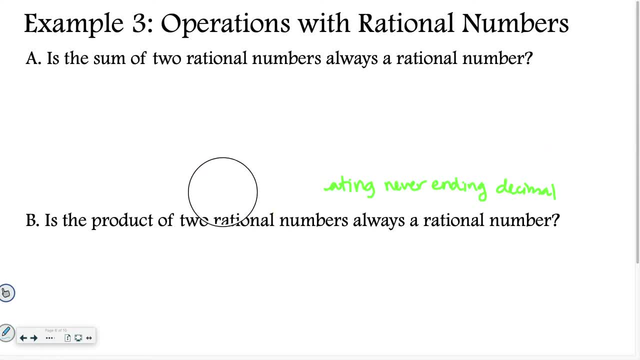 Is the sum of two rational numbers always a rational number? So let's think about that. Two rational numbers. We said any rational number can be written as a fraction, right? So what if I did like 1 eighth plus 2 eighths? 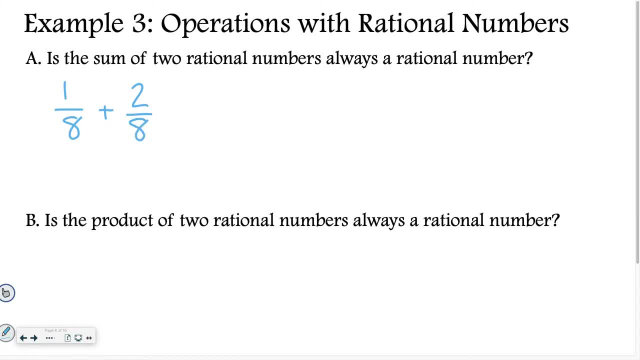 Okay, so that's two rational numbers, right? They're two fractions. Well, the sum of those would be 3 eighths. Okay, so 1 eighth plus 2 eighths is 3 eighths, and that is a rational number, right. 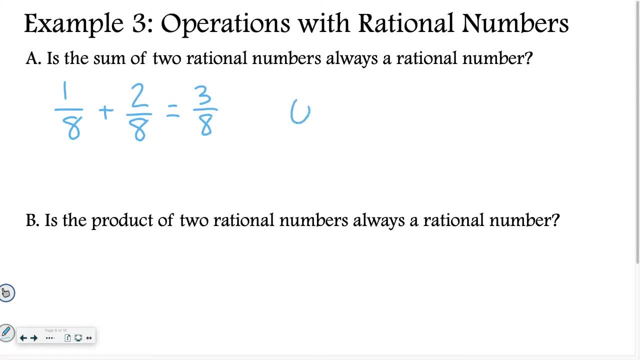 Because it's another fraction. What if we did like 0.45 plus 0.3?? Those are both rational numbers, They're decimals that end right, And it would be 0.75,, which is another rational number. 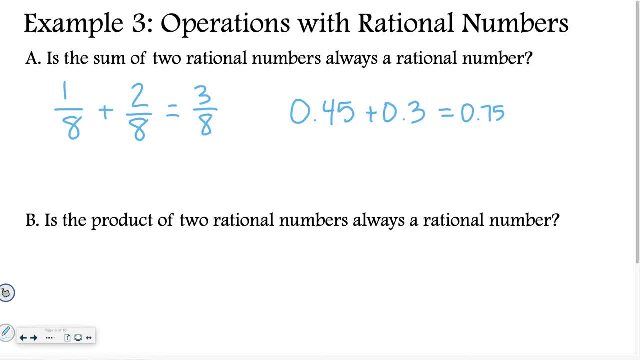 So the sum of two rational numbers. I'm not going to get into a big long explanation about this, but two rational numbers, when you add them together, will always be rational. okay, The sum of two rational numbers is always rational. 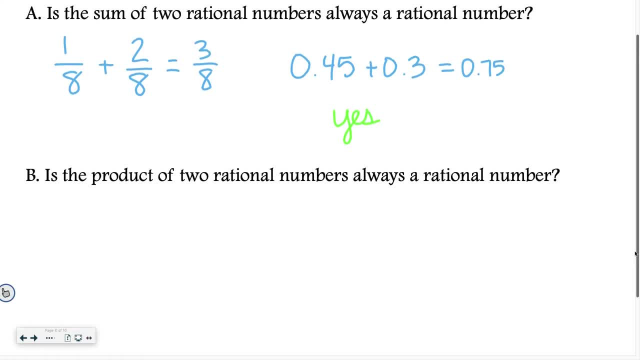 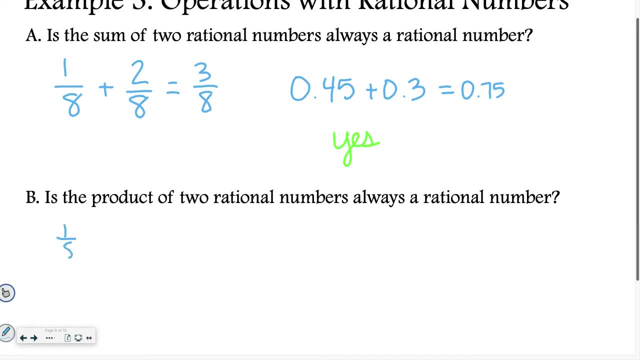 Then letter B. what about the product of two rational numbers? So let's try the same thing. If I did 1 eighth times 2 eighths, if I multiply those, I would have 2 sixty-fourths or 1 thirty-second. 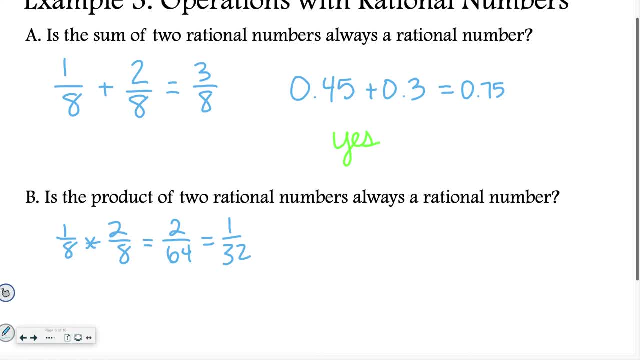 Well, that's still a fraction, so that is still a rational number. And I could do 0.45 times 0.3, and I end up with 0.135, another decimal that ends right. So the product of two rational numbers. 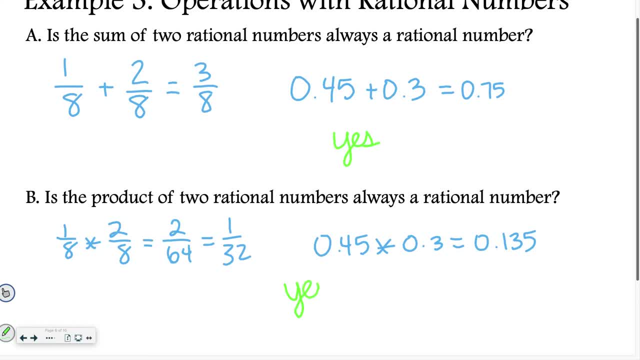 again. I could go into a big long explanation, but this is a point where I'm telling you to trust me, I'm not going to expect you guys to know the next level of thinking with this. okay, So the product of two rational numbers is always a rational number. 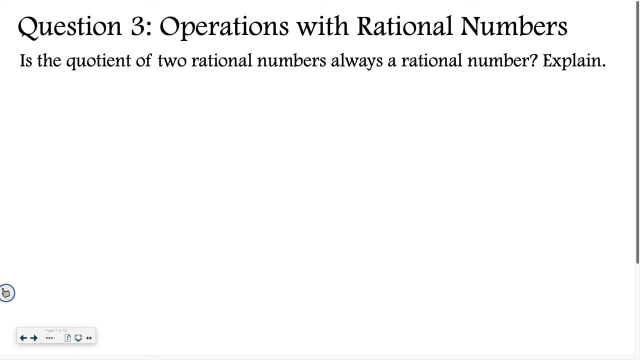 Question number three- This one's for you- Is the quotient of two rational numbers always a rational number? Explain, Good luck, Hopefully. the answer you said is yes. I wrote out one example right. So the quotient means we're dividing. 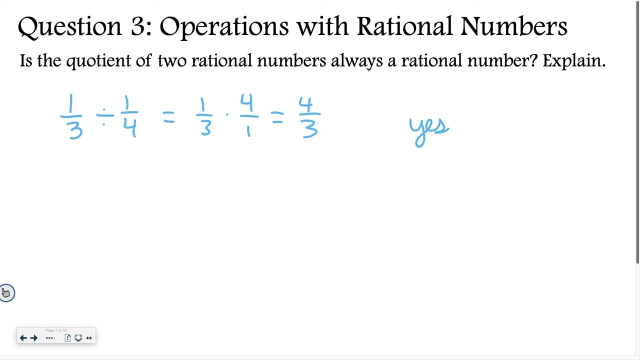 So what if I divided two fractions? Because we've already said that fractions are rational. So 1 third divided by 1 fourth. Well, if I'm dividing fractions, that is the same as multiplying fractions or multiplying by the reciprocal right. 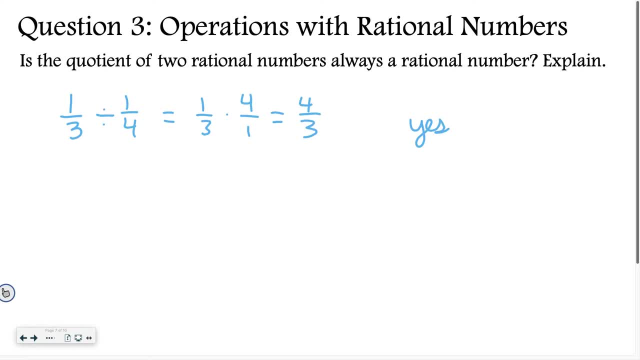 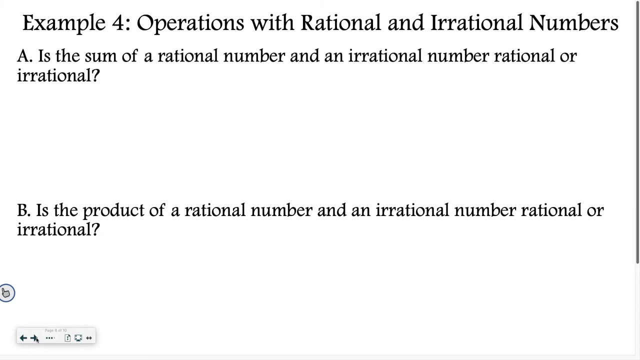 Which means that I'm multiplying two rational numbers, which on the last slide we said is rational. So your answer would be yes, All right. Example four Is the sum of a rational number and an irrational number rational or irrational? So let's think about that. 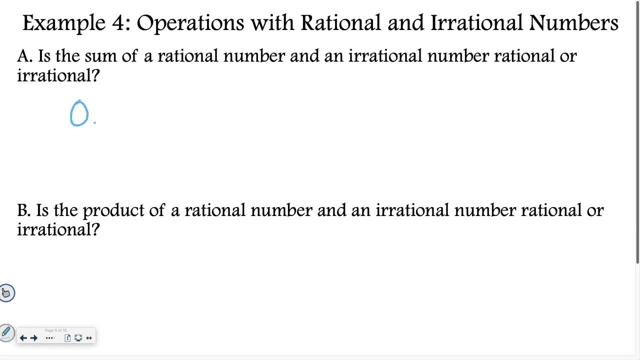 This is sometimes easier with some decimals, So I'm going to just choose 0.25.. And why don't we say plus pi? Okay, So I'm going to add pi to this right, Plus 3.141592653.. 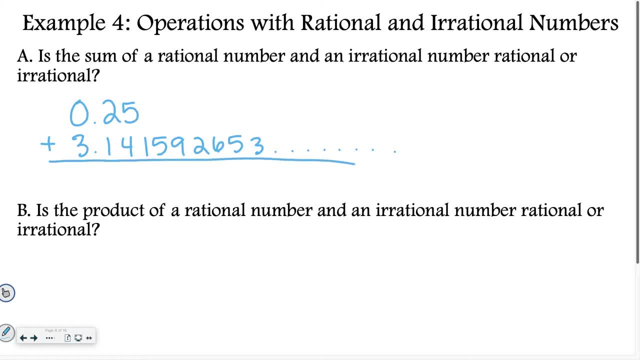 These numbers are going to go on forever and ever, right? So just because I add 0.25 to it, these numbers over here after this 5 are just going to stay the same and continue on forever and ever. They're not going to repeat. 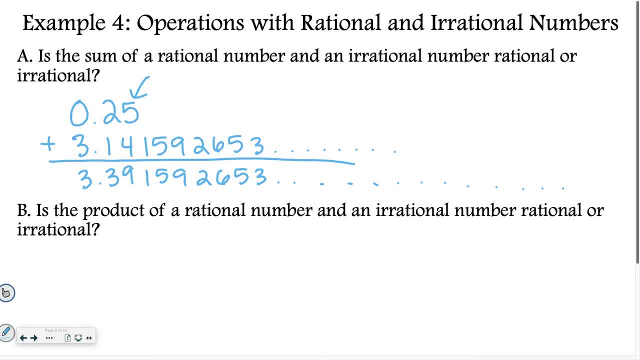 they're not going to end. So when you add a rational number to an irrational number, it's still going to be irrational because the irrational number is going to go on forever and ever beyond the end of that rational number. So then, letter B is the product of a rational number. 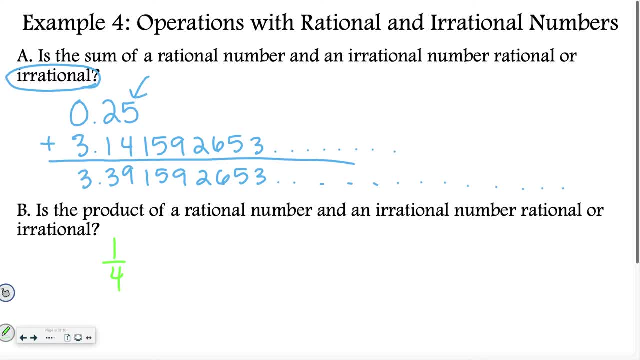 So let's try that. And an irrational number? rational or irrational. So if I did 1 4th times, let's see. thus we'll do pi again because we like pi. Okay, So if I did 1, 4th times, pi. 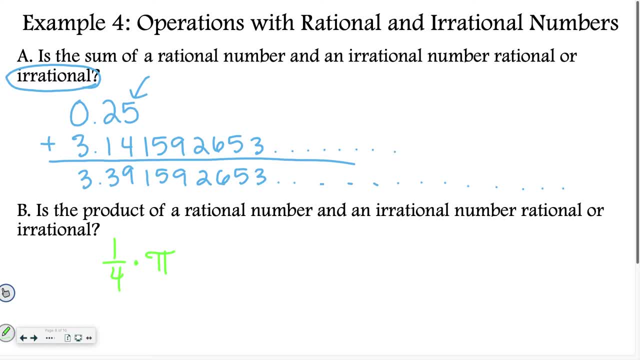 I'm still going to have a big long decimal. that continues on and on and on And it keeps going forever and ever, Because that's how pi works. So when you multiply a rational and an irrational number, you end up with an irrational number. 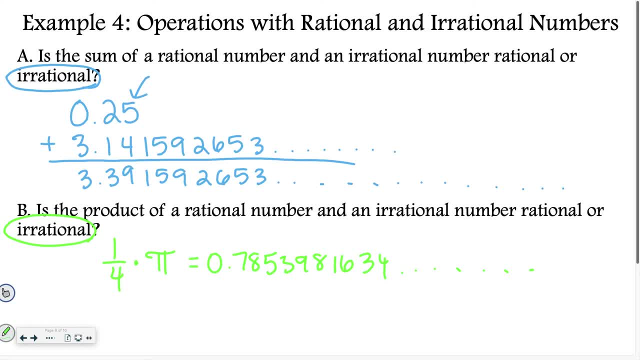 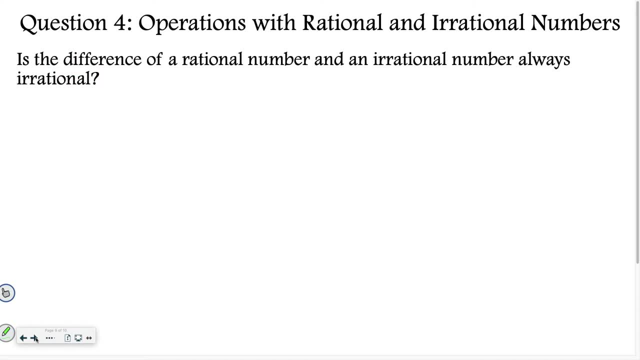 Okay, So that is important for you to remember. The next question is for you: Is the difference of a rational number and an irrational number always irrational? Good luck. Hopefully you answered with yes And you may not have an idea of why you said yes. 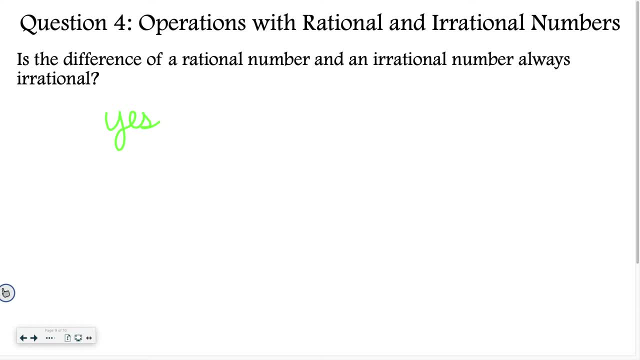 You might be like getting really excited in front of your laptop because you just guessed yes and you happened to be right. But let me tell you the rationale behind why the answer is yes. So on the last or a couple slides ago, we talked about how 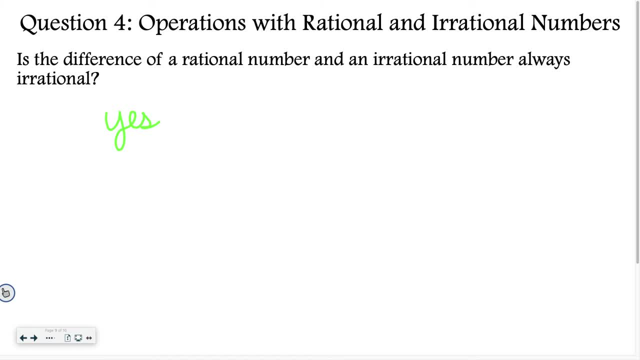 or on the last slide, we talked about how the sum of a rational and an irrational number was irrational. Now, if we think about difference, difference is the same as sum, except one of your numbers is negative. Right, So you can think of subtracting as adding a negative number. 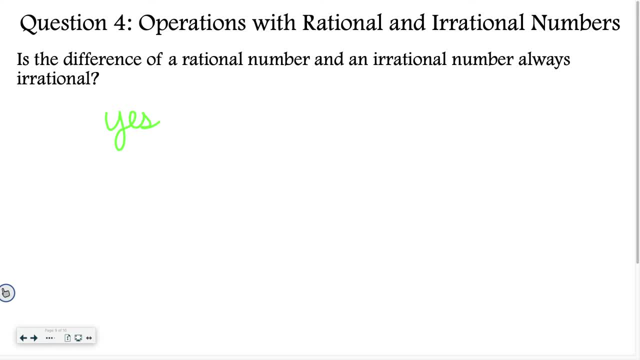 So really difference? this operates the same way as a sum. When you add a rational number or when you subtract a rational number and an irrational number, you're going to have an irrational number. You're going to have a number that goes on forever and ever. 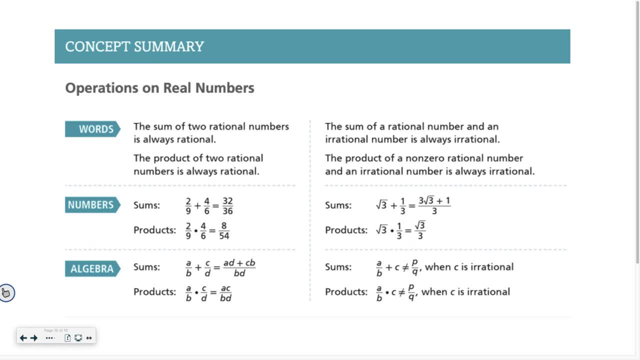 Okay, And this last slide, the concept summary, summarizes everything in one nice slide for you. So if you're someone that struggles to take notes but likes to reference things, if you take a screenshot of this slide, this slide will be your best friend for this section. 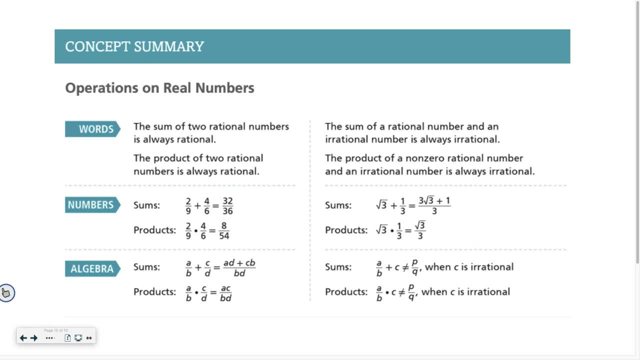 It summarizes everything you need to know. I will tell you that if you're looking at this slide, this bottom portion here is the stuff I didn't cover in this video. That doesn't mean that you can't look at it and you can't learn about it. 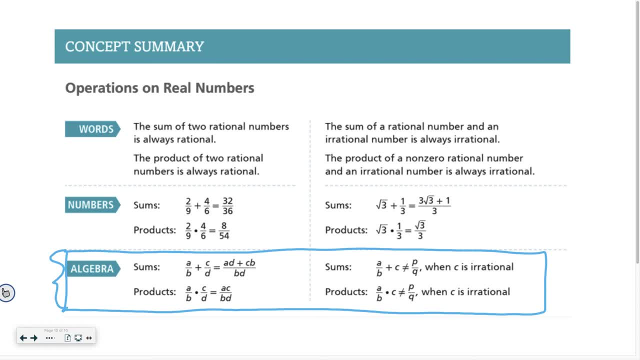 That is the next level for those of you that want to go to that next level, And we can certainly talk about that one on one. But I'm not going to test you on this kind of stuff. I will test you on this stuff up here. 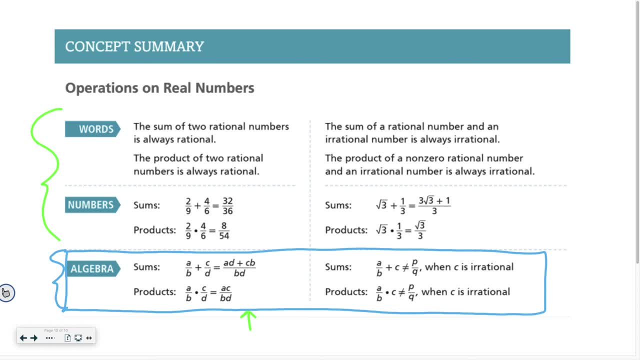 That's what we talked about in today's video. If you have any questions at all, please be sure to reach out for some help, and I'd be more than happy to assist you. Have a great day.